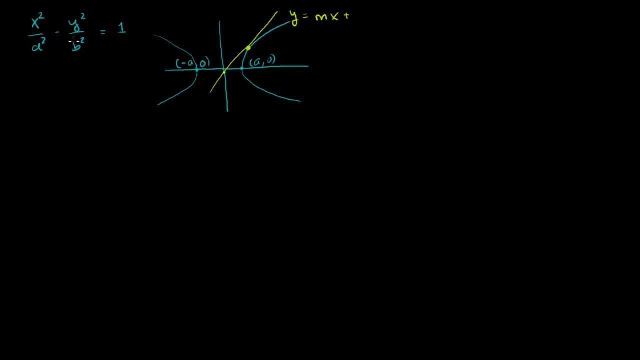 so normally we would call the y-intercept b for a line. we've already used the b here in the equation for the hyperbola, so let me just call this c. So the c is a little unconventional. This is going to be the y-intercept. 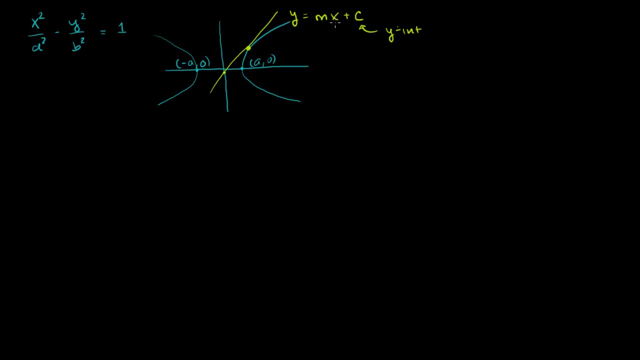 So let's see if we can come up with a relation between these two, Between the m's, the c's and the a's and the b's. And we already used it in one of the IIT problems And I suspect that the next one I'm 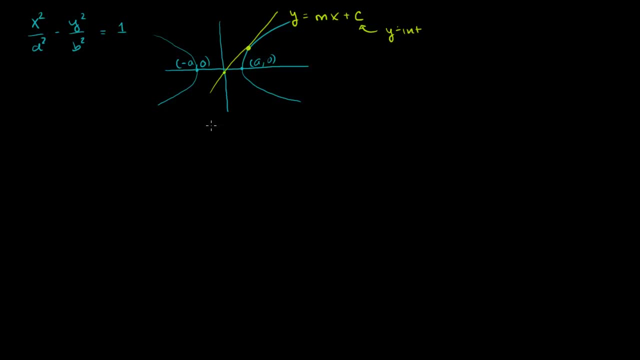 going to do will also use this, And if y'all have seen a lot of Khan Academy videos, you know that I always like to prove things from first principles, Because in life you can't just memorize formulas: You won't know where they came from. 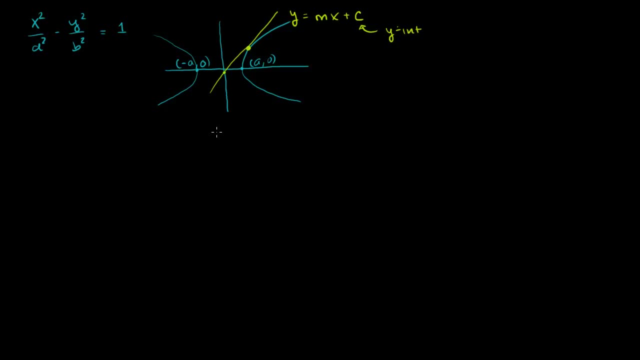 You'll memorize them wrong. You won't understand what they actually mean. But if you're going to take the IIT JEE exam, I would recommend that you, because I've I have appreciation for how little time they give these problems. 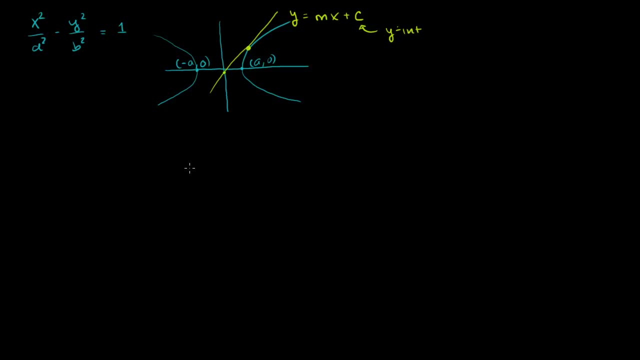 And if you have to prove from first principles, you won't be able to prove them. So let's just come up with a relation. Let me stop talking without drawing. So let's just see where they intersect, And the whole insight here is that they're only 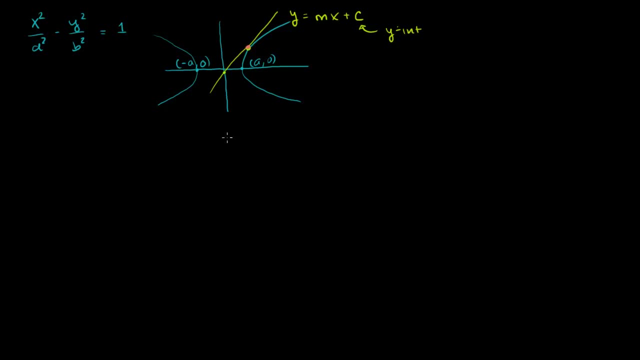 going to intersect in one point. So what I'm going to do here is solve for y squared. So over here we can multiply both sides of this equation by: let's multiply both sides by negative, Negative b squared, And so you get negative b squared over a squared. 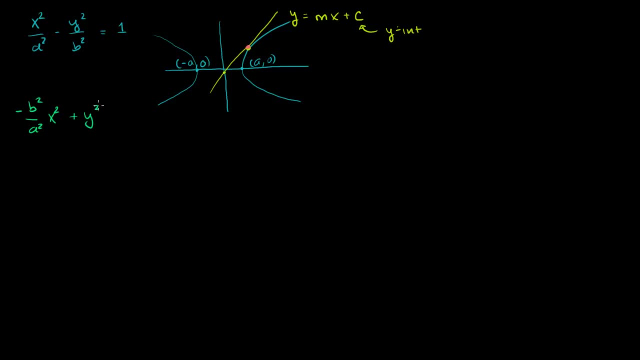 x squared plus y squared, right I multiplied by negative b squared is equal to negative b squared. And now let's add this thing to both sides of this equation And we get: y squared is equal to b squared over a squared. 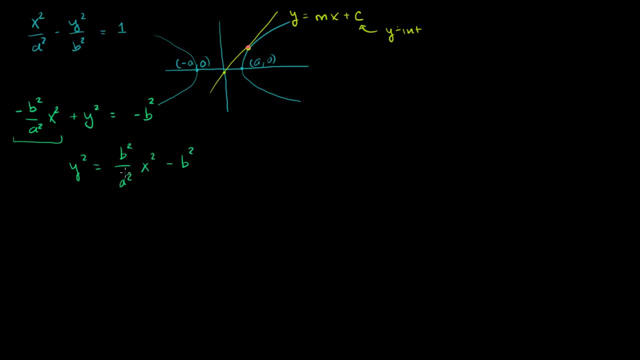 x squared minus b squared. So I just rewrote the equation for the hyperbola, And let's also write this in terms of y squared, And then we can set them equal to each other. So over here, in this greenish, yellow-like color. 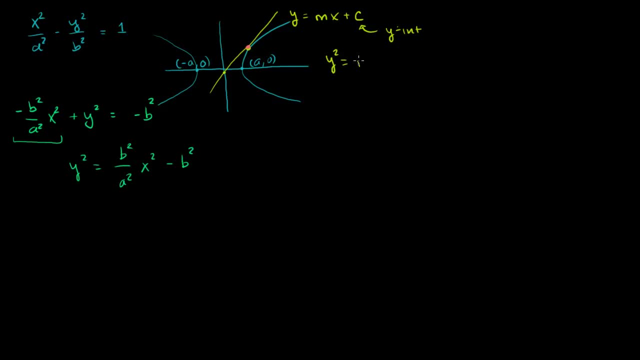 if we square both sides we get: y squared is equal to m squared, x squared plus 2 times the product of both terms, So plus 2mcx plus c squared. So in order for them to intersect, they both have to be at the same place at some, x and y. 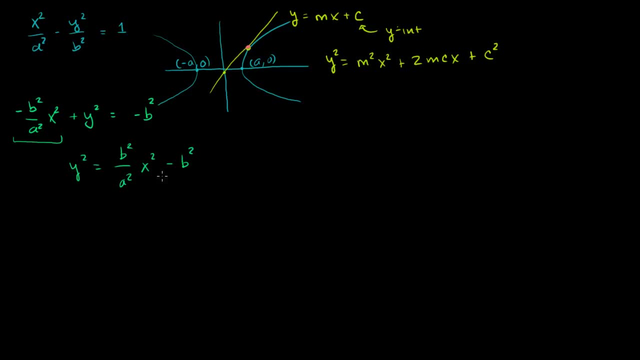 So we can set this y squared being equal to that y squared and then try to solve for the x. Obviously we won't be able to solve for the x because there's so many variables. We can find a relationship between this a, this b. 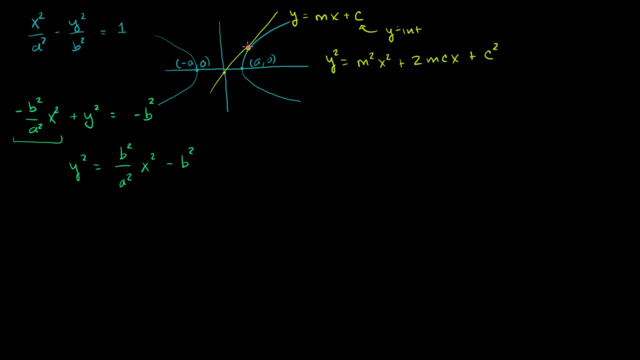 this m and this c, So there's only one point of intersection, which, by definition, it would have to be at the tangent point. So let's do that. So we have m squared, x squared plus 2mcx plus c squared. 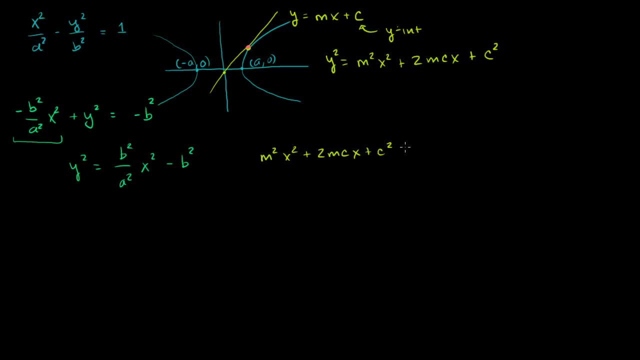 Plus c squared is equal to b squared over a squared, x squared minus b squared, And I've done a very similar exercise to this in a previous IIT-JE video. But here I just want to focus just on the most general case. 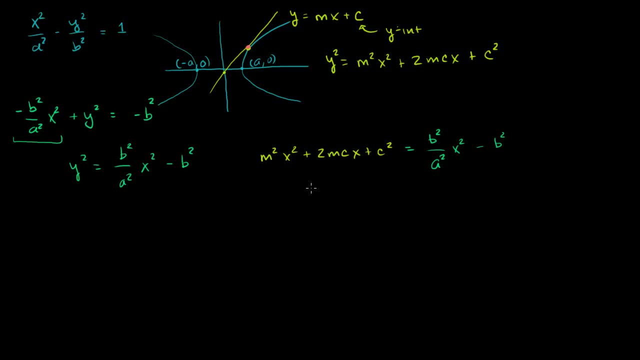 so that we have something that we can add to our toolkit. So let's write this in terms of a quadratic equation in x. So if we subtract this from both sides, we get m squared x, We get m squared. We have m squared minus b squared over a squared x squared. 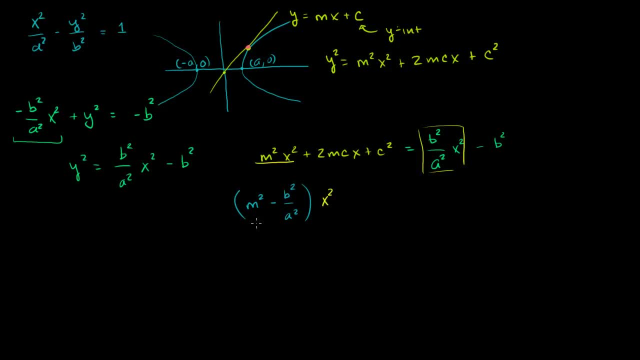 So that's that term and that term right over there. And then my only just first degree x term is right over here. So plus 2mcx, I'll write it in- plus 2mcx And then finally plus 2mcx. 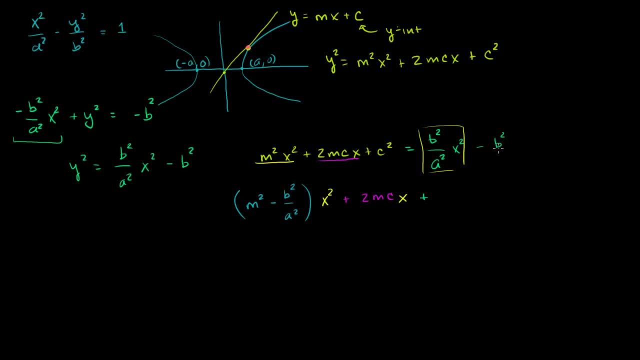 Plus we have a c squared, And then we're actually going to have a plus another b squared over there. So this is going to be plus c squared, plus b squared. Now, in order for this equation to only have one solution, let me write down: this is going to be equal to 0.. 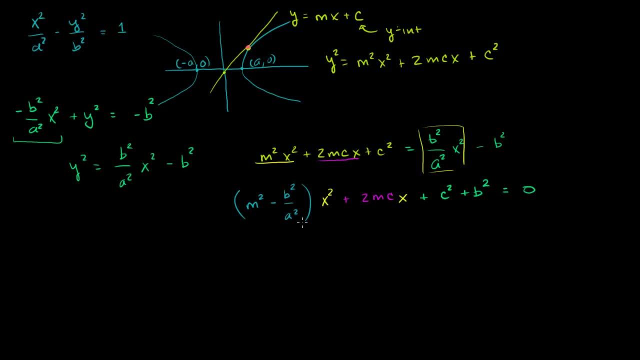 In order for this thing to only have one solution: the discriminant of this equation. let me write down this. So I'm going to write this down. So let's write this down. Let's say: I have a quadratic equation. Remember, when you do the quadratic equation, 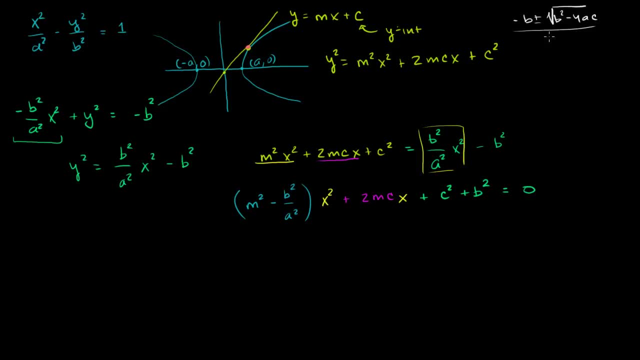 and these are completely different. so negative b plus or minus the quadratic formula b squared minus 4ac over 2a. You're only going to have one solution if this thing over here, if the discriminant over there is equal to 0.. 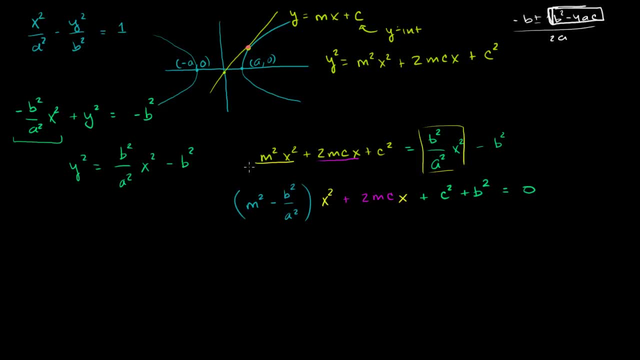 If b squared minus 4ac is equal to 0, then you only have the solution negative b over 2a. So in this situation, for the tangent line, you can only have one solution, One x that satisfies this equation. 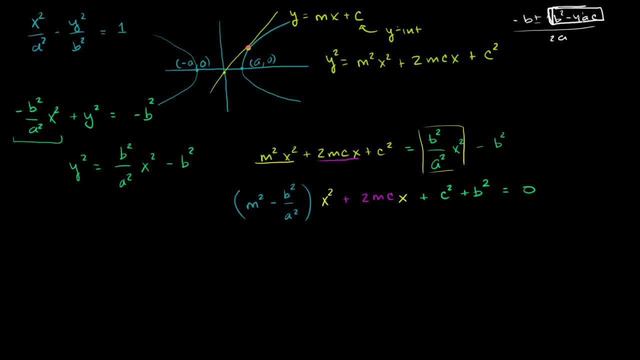 So b squared minus 4ac is going to have to equal 0 in the quadratic formula. These are different b's and a's and c's than the ones we're using here Over here. our b is that right over there, the coefficient on the x term. 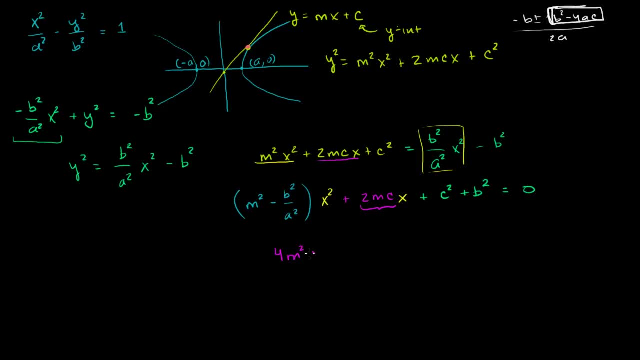 So that squared is 4m squared, c squared, And we're going to subtract from that minus 4 times a. a is all of this. It is all of this business right over here, And just to simplify things, let me make this plus. 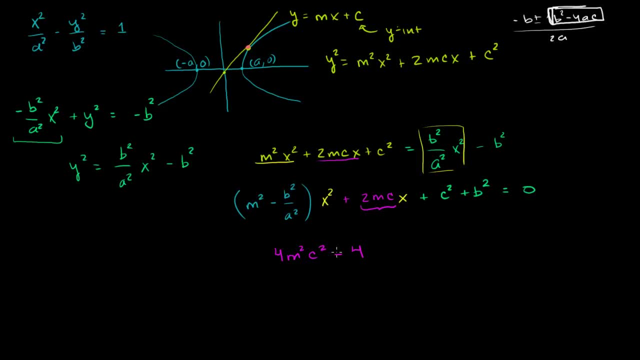 and then multiply this times a negative sign and it'll reverse the sign. So I'll put minus 4, I'll put a plus here times instead of writing, since I have to multiply this by negative 1, it'll now be b squared over a squared minus m squared. 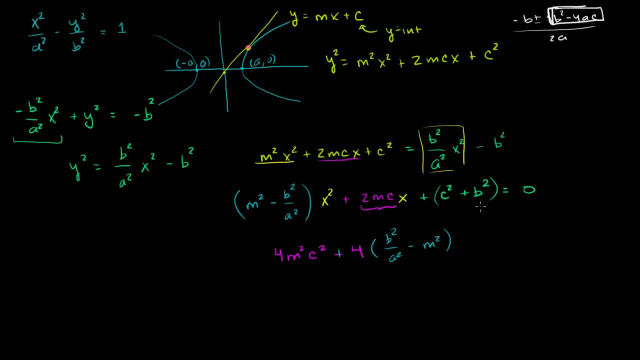 And then the c is this term right over here. This right here is c 4ac, c squared plus b squared, And this thing is going to equal 0.. It's going to equal 0 if this line is tangent, if we only have one solution. 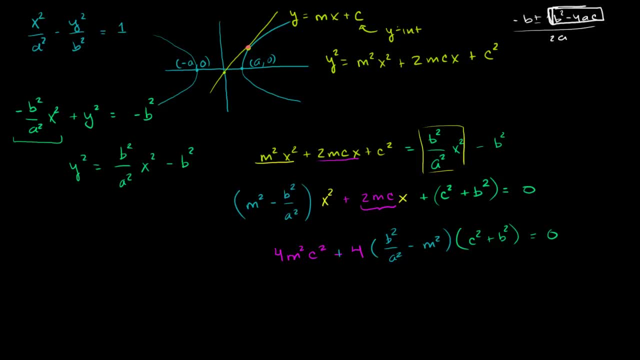 So let's see. the first thing that we can do to simplify this is: we can divide both sides of this equation by 4.. And if we do that, this becomes a 1.. So we can ignore that, and then this becomes a 1.. 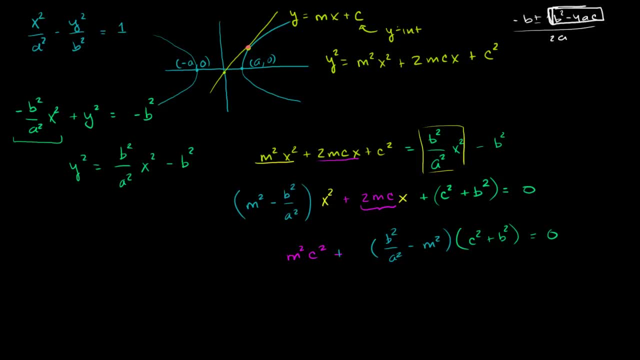 So that simplified our equation a good bit. And now let's multiply the second part right over here. So we have b squared over a squared times c squared. That is b squared, c squared over a squared, And then b squared, a squared times b squared. 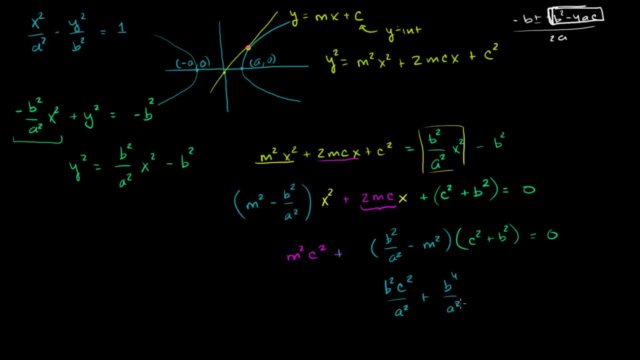 So plus b to the fourth over a squared, And then you have negative m squared times c squared. So let me do this in another color. So then you have negative for the m squared, Negative m squared, c squared, And then you have negative m squared, b squared.